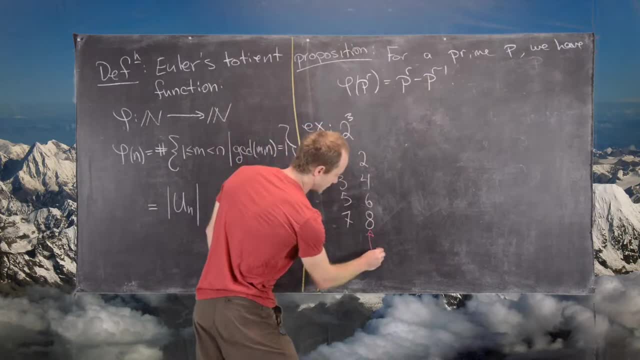 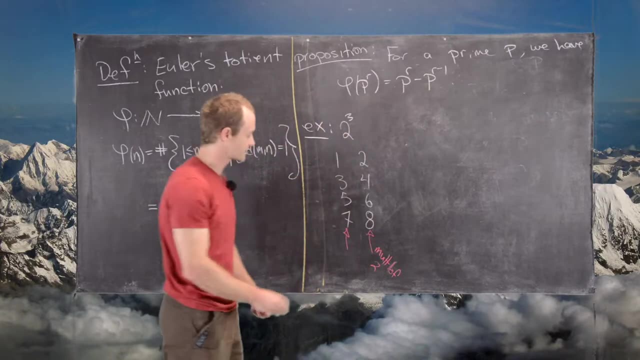 in my last column. so I'll do 1,, 2,, 3,, 4,, 5,, 6,, 7,, 8.. And so the way that I will do that is is a multiple of 2, which makes everything in my first column relatively prime to 2.. 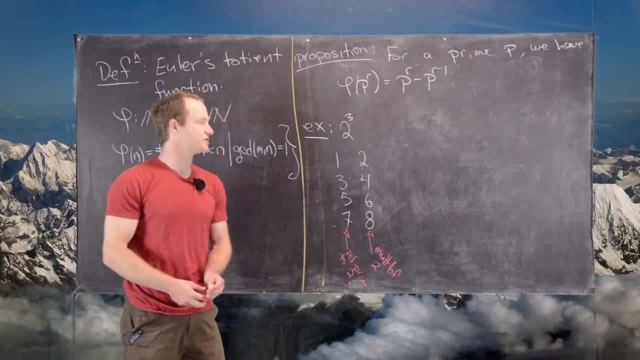 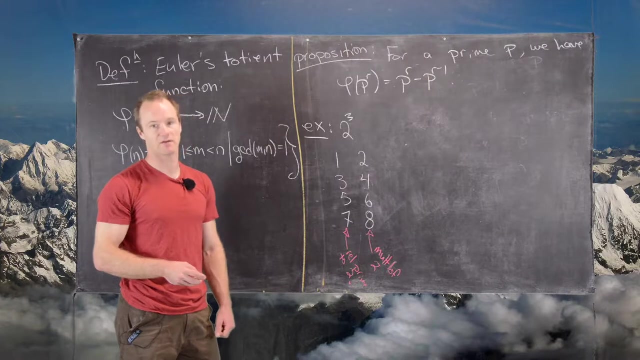 And so since it's relatively prime to 2, that means it also has to be relatively prime to 2 cubed. In fact, if something is relatively prime to a power of a prime, then it has to be relatively prime to that prime, and vice versa. So now notice. what we get here is we can count up 1,, 2,, 3,, 4.. 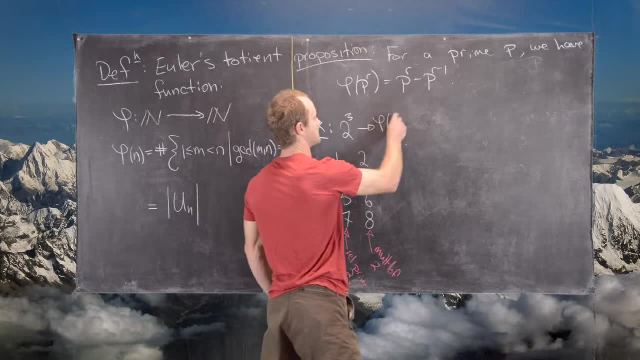 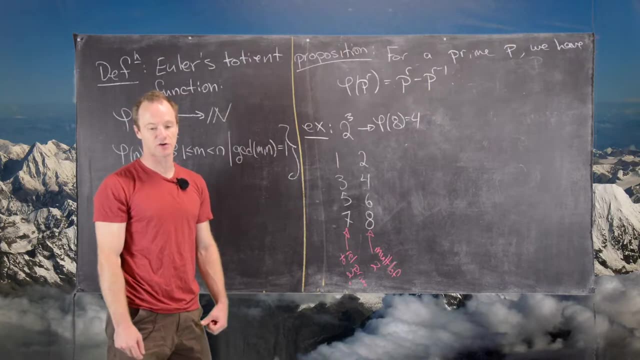 Good. So that tells us that phi of 8 equals 4.. So maybe this doesn't give us some insight into the proof in general, but maybe if we do one more example we'll have some insight. So let's look at 3 squared. 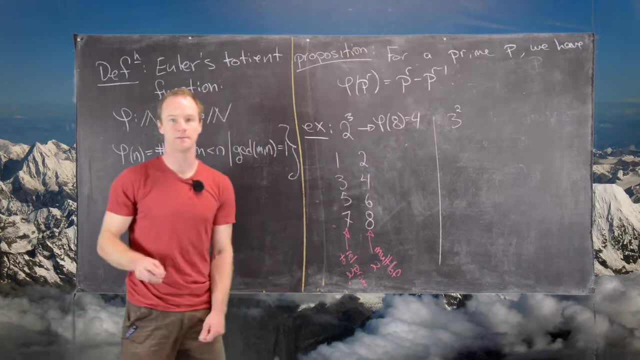 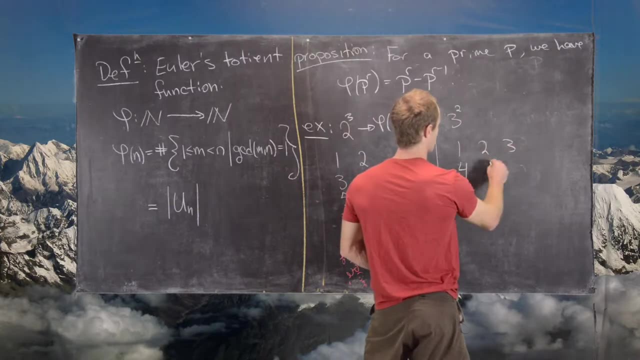 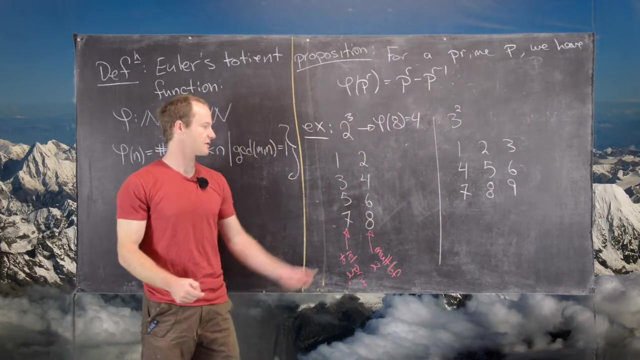 So if we have 3 squared, which is obviously 9.. So again I want to make an array, So 1, 2, 3, 4, 5, 6, 7,, 8,, 9.. So now I have an array and it's a little more interesting. 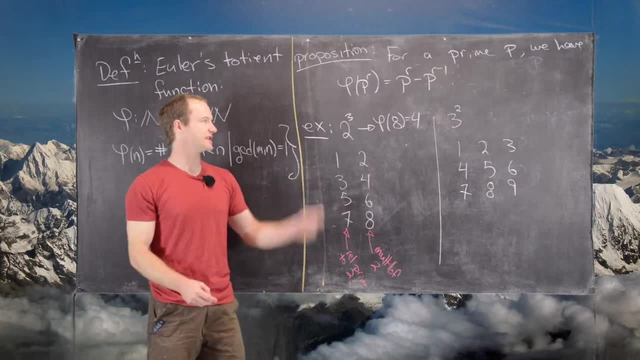 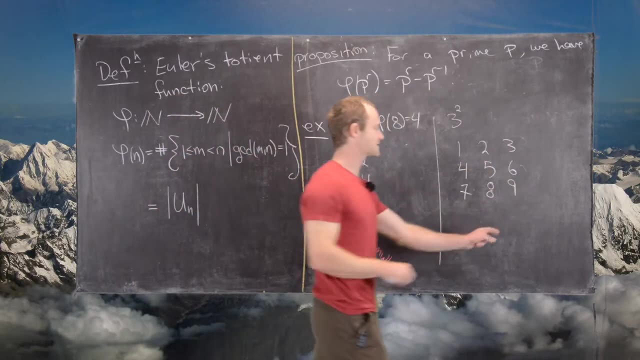 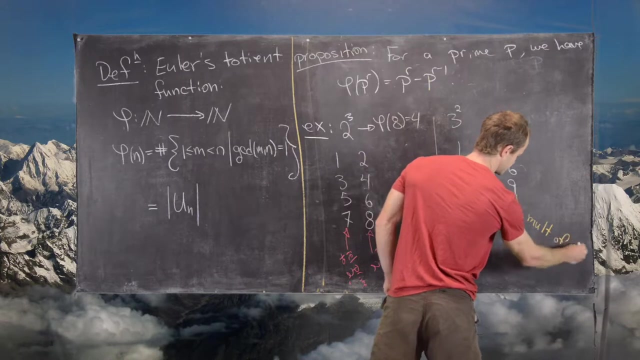 because it has 3 columns instead of 2 columns. And now, notice, in general, I'm going to have p columns where p is my prime. And now, notice, on this last column, we have all of the multiples of 3.. So those are all of the multiples of 3.. And if you are not a multiple, 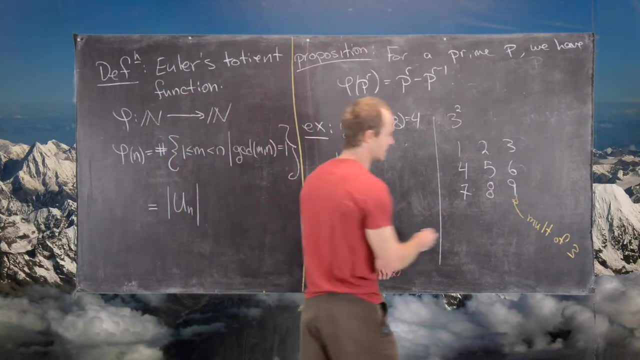 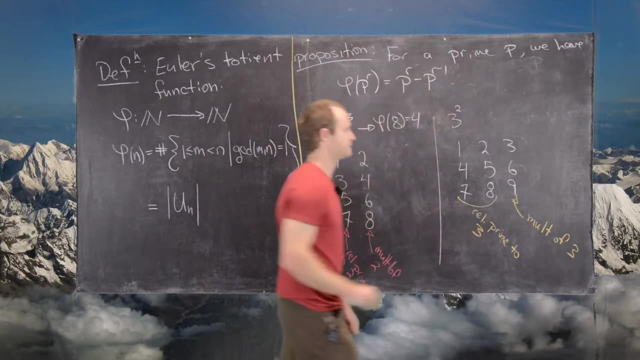 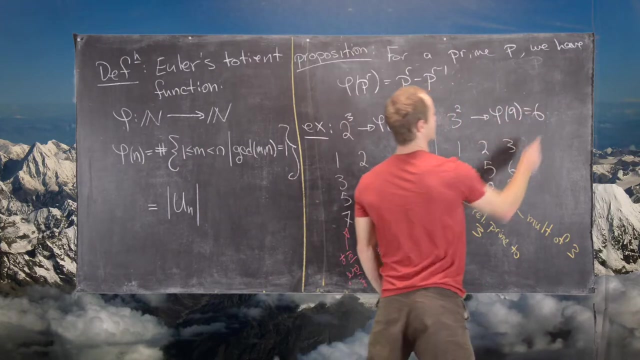 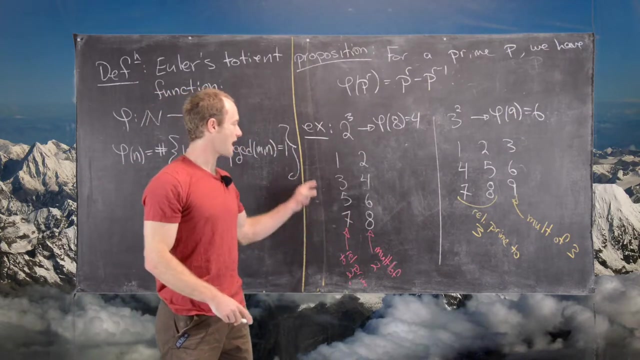 of 3, then you can't be relatively prime to 3.. So that tells you that everything over here is relatively prime to 3.. Great. So now notice, that tells us that phi of 9 equals 6.. So let's see what's really going on here. So now notice, in this case we made an array. 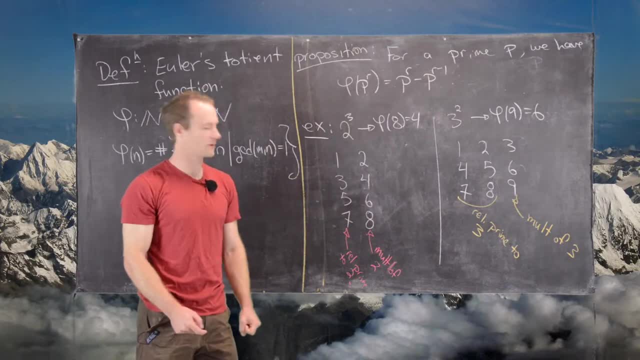 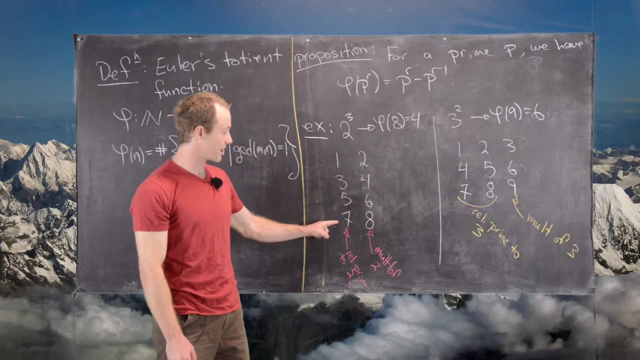 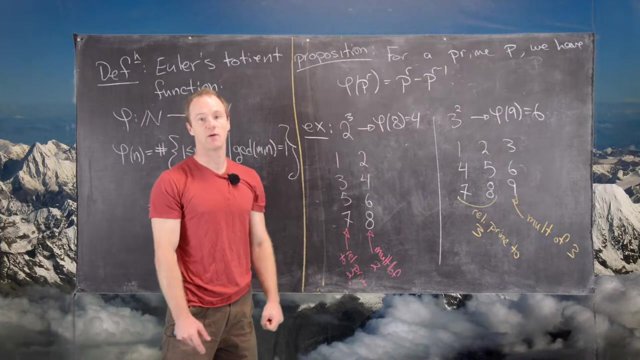 that was 2 by 4.. And the last column was a multiple of 2.. The first column was everything relatively prime to 2. So in fact we're taking kind of the area of this subarray that's left over after we delete everything. that's a multiple of 2.. Now in this next example, 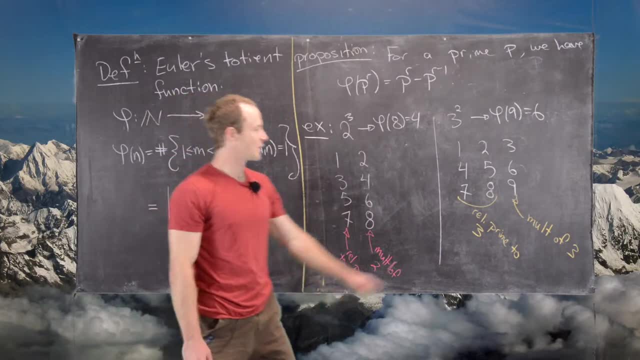 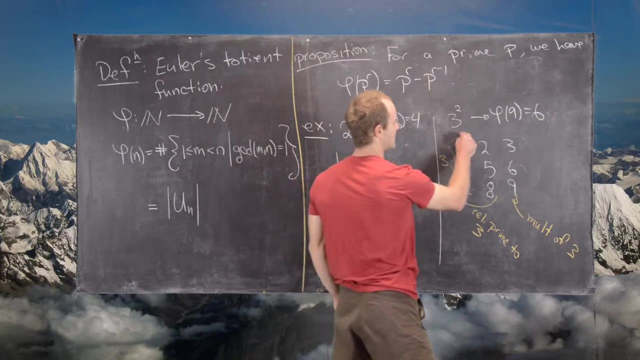 we're making an array that's 3 by 3.. We're taking off the multiples of 3.. And now notice what's left is an array which is 3 by 2, which is 6.. And so that'll be the motivation for. 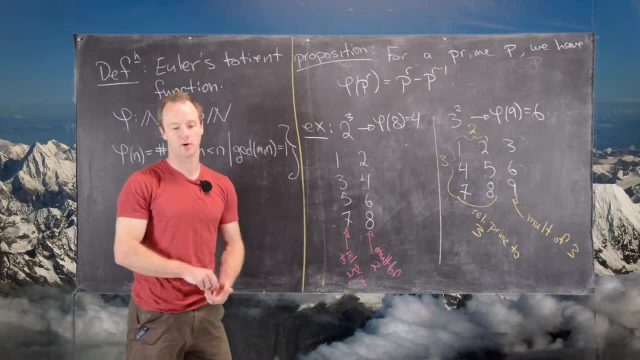 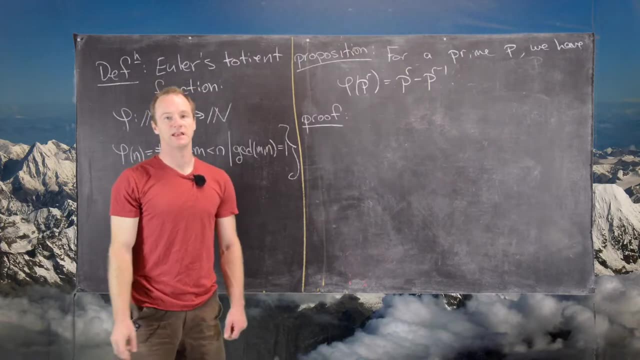 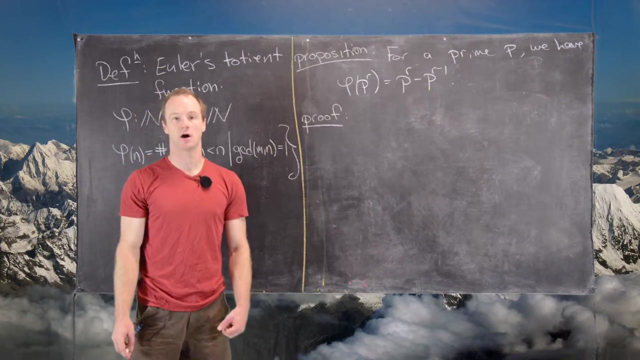 the general proof, as we'll see once we clean up this board. Okay, good, So I'll clean up the board and then we'll look at this generally. Okay, now we're ready to look at the proof in general. So we have a prime p and we're looking at a power p to the r. So what we want to do, 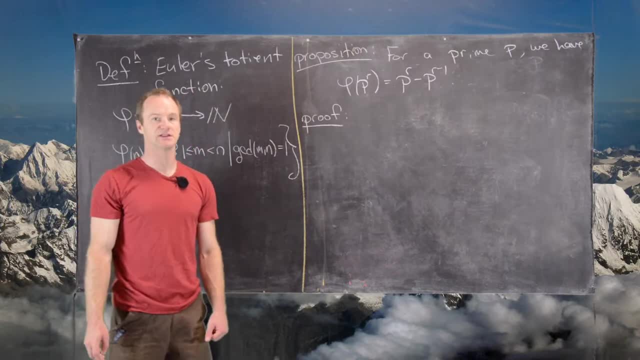 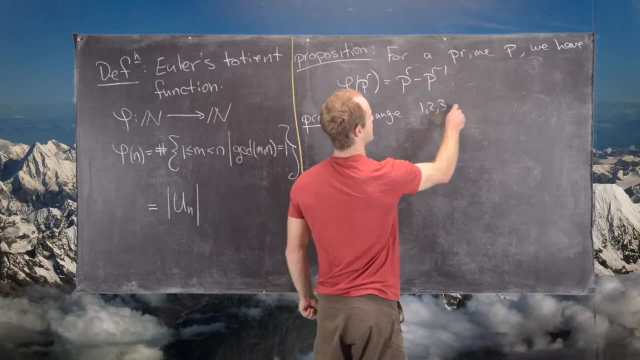 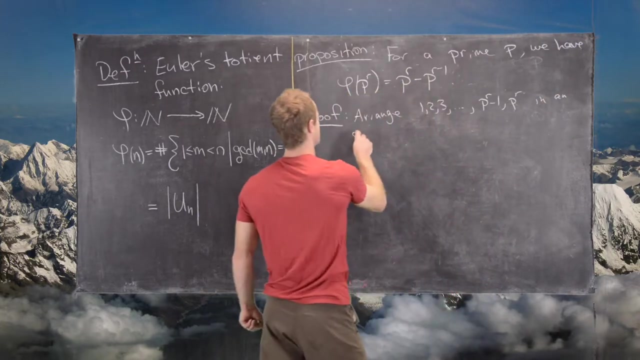 is lay out all of the numbers 1 to p to the r in an array. So let's arrange 1, 2, 3, all the way up to p to the r minus 1 times p to the r in an array as follows. So we'll do. 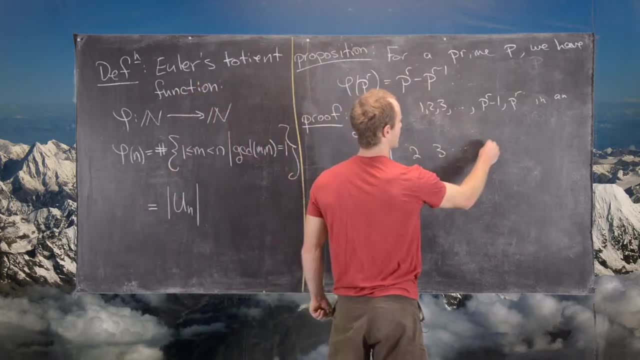 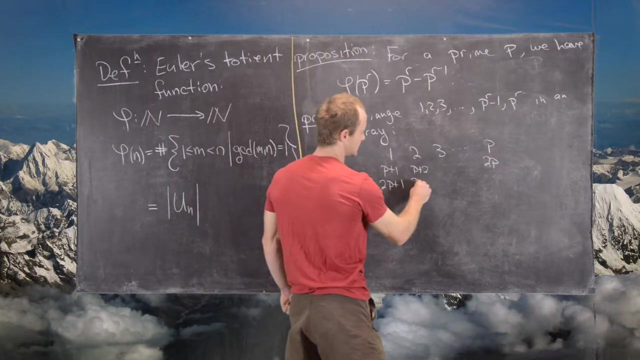 it like this. So this is going to be 1,, 2,, 3, all the way up to p, and now this is p plus 1,, p plus 2,, all the way up to 2p. And now the next thing will be 2p plus 1,, 2p plus 2,, all the. 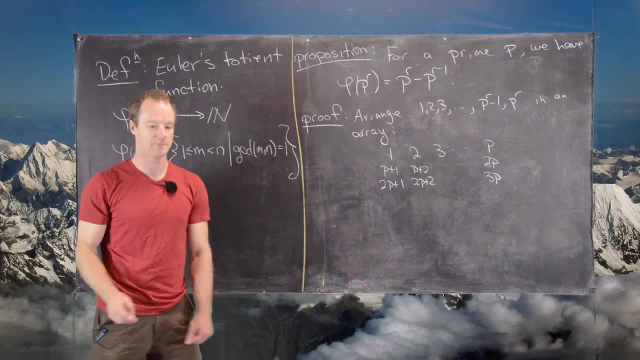 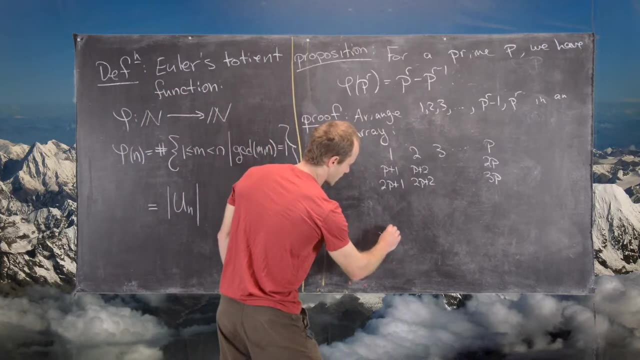 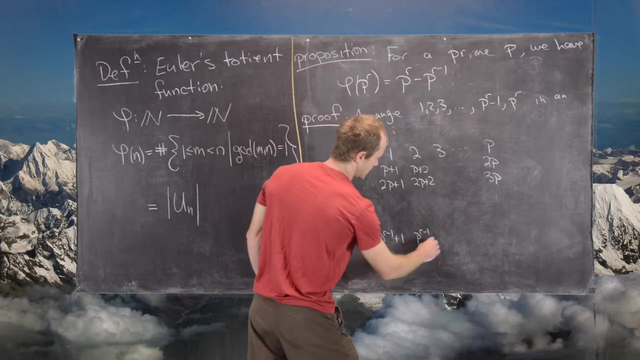 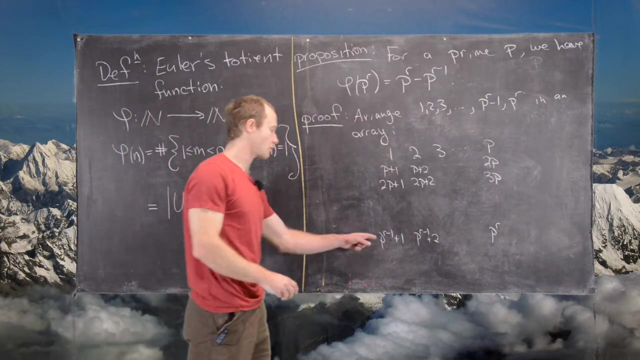 way up to 3p. Good, And then, finally, at the end, we will have p to the r minus 1 times 2p plus one, p to the r minus one plus two, all the way up to p to the r. Great, Now, if we wanted to look. 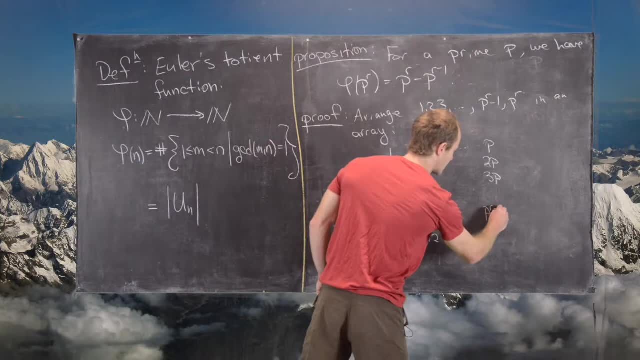 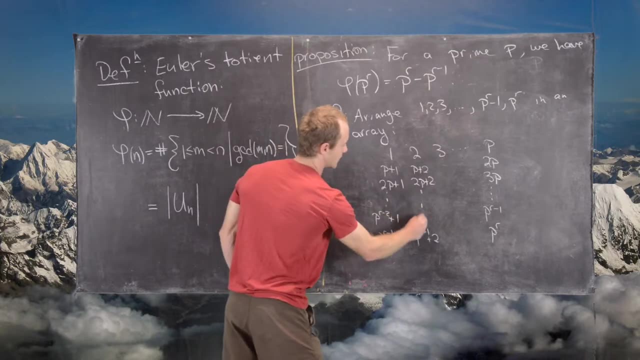 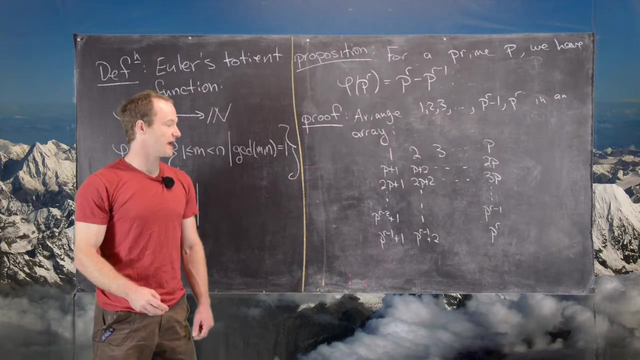 right above this. this would be p to the r minus one, and now this would be p to the r minus two plus one, and so on and so forth. So this is the structure of our array. Good, So now what we can see is of all of these numbers laid out in this array. 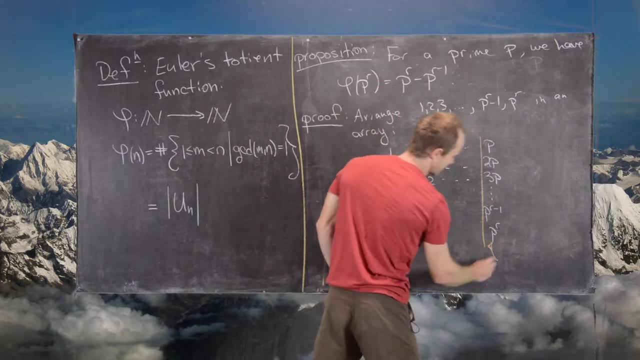 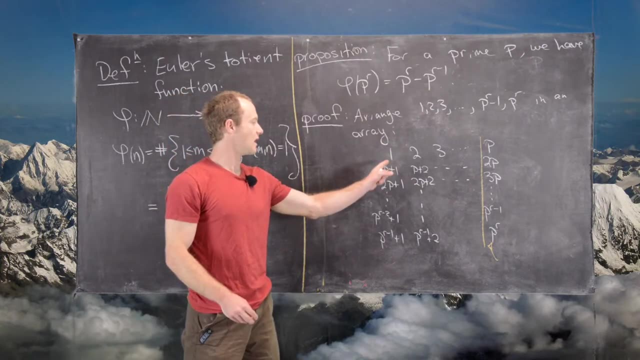 this column, at the very end, is the only thing that is not relatively prime to p. And we can see that because everything here is given by, you know, taking the quotient with p and then looking at its remainder. So everything here has a remainder. 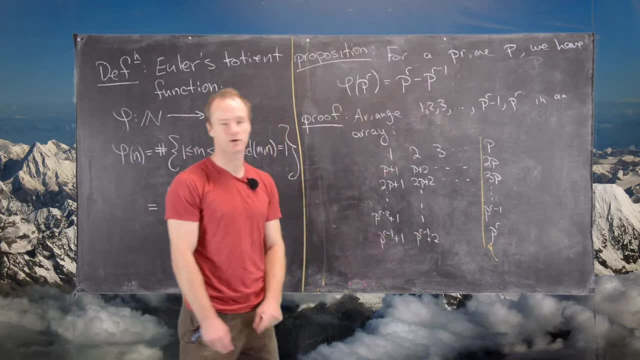 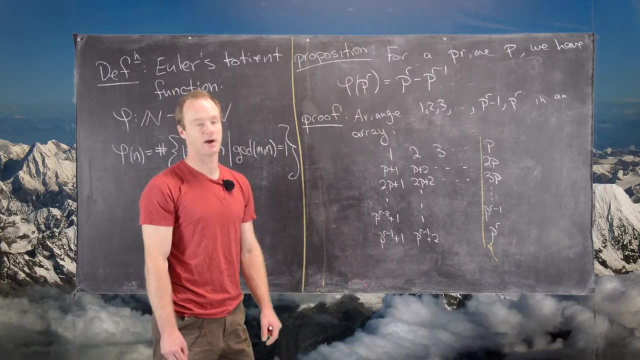 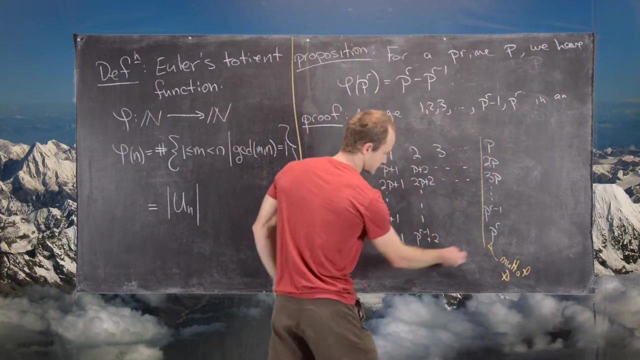 of 1 when divided by p. Everything here has a remainder of 2 when divided by p. And all the way up here, everything down here, has a remainder of p minus 1 when divided by p. So over here, these are all multiples of p, And then, over here, this is everything that. 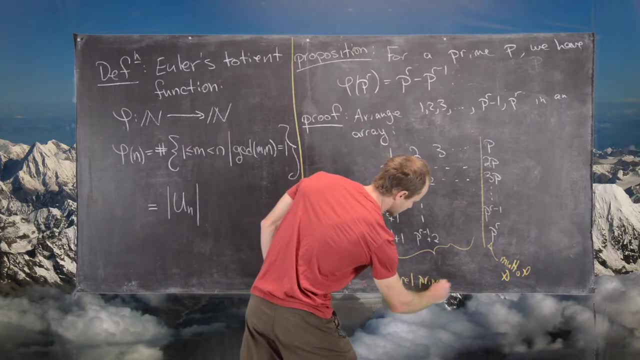 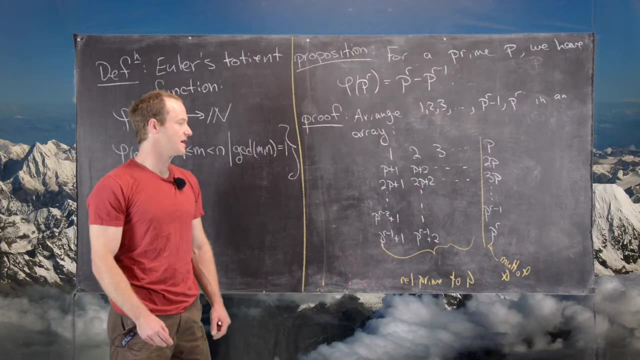 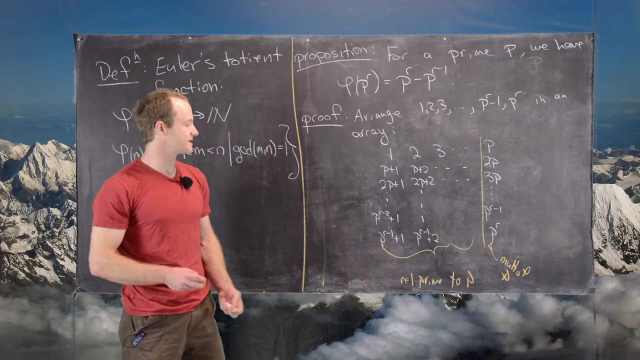 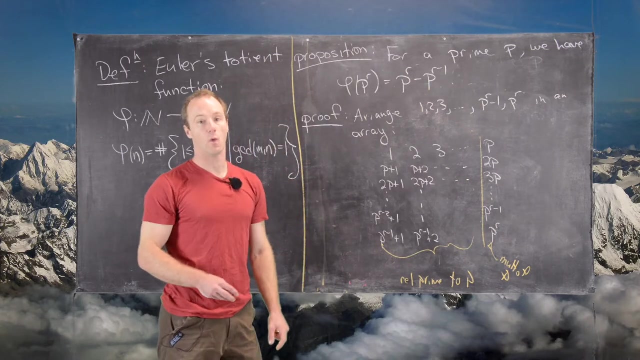 is relatively prime to p. And now, since we've arranged this as an array, all we have to do is find the height and width of this array. So let's see if we can do that. So now notice this is going to be. the total array is 1 to p wide, So that means what's left over. 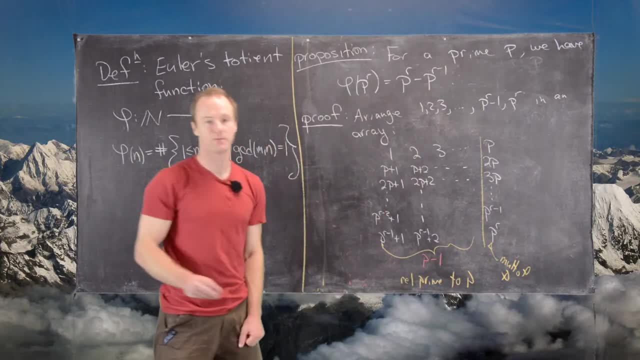 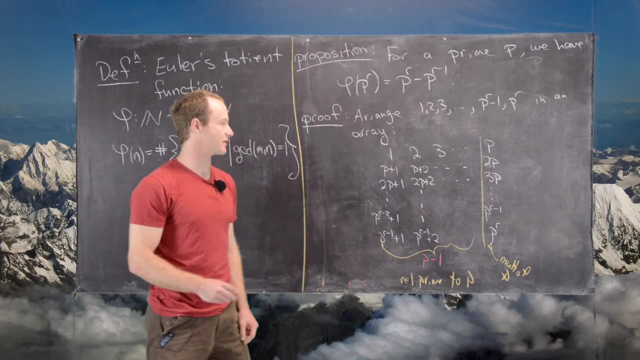 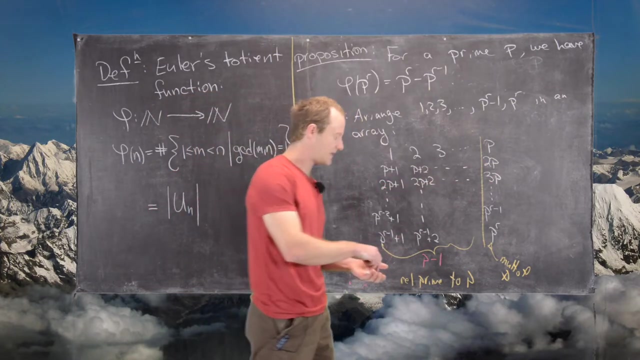 is p minus 1.. So we have p minus 1, numbers running the width of the array. And now let's look at the height of the array. So notice, we have 1 times p, 2 times p, 3 times p, And then, if we view, 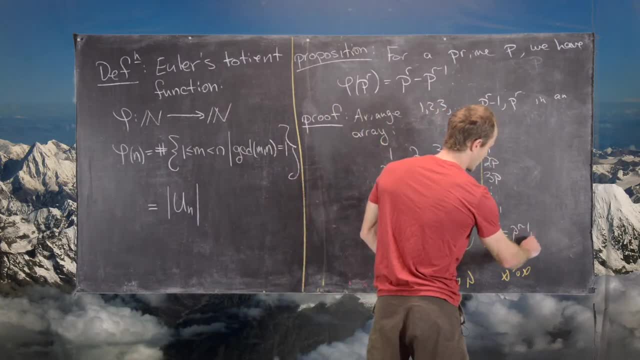 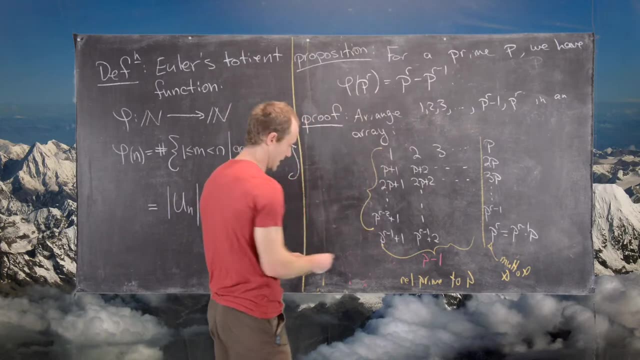 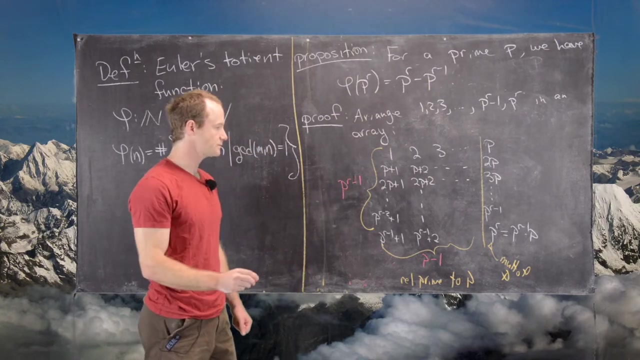 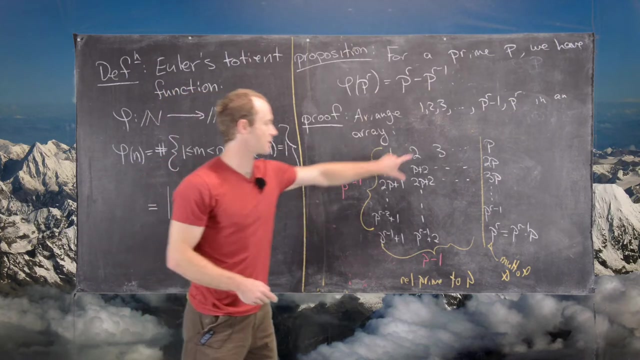 this number down here as p to the r minus 1 times p, we can see that the height of the array is given by p to the r. Good, So now, all of those things that I've just said, allow us to count up the numbers. 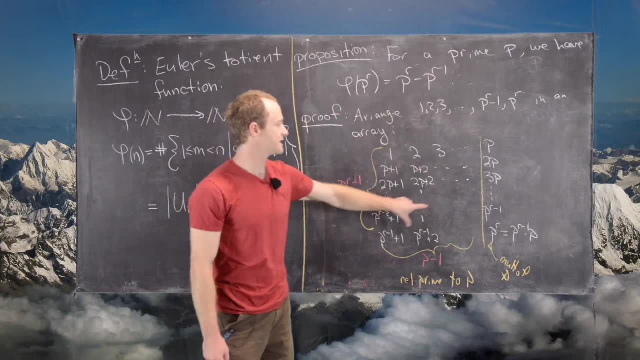 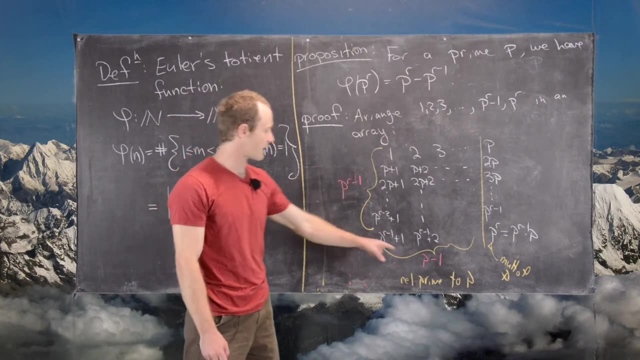 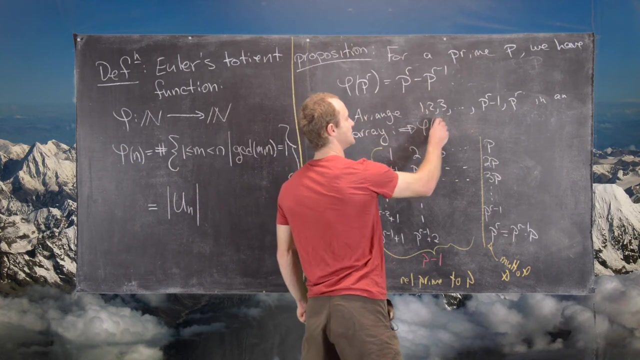 in this portion of the array. So the numbers in this portion of the array which give us all the numbers relatively prime to p to the r, so that will be p minus 1 times p to the r minus 1.. So again that tells us that phi of p to the r is p to the r minus 1 times.